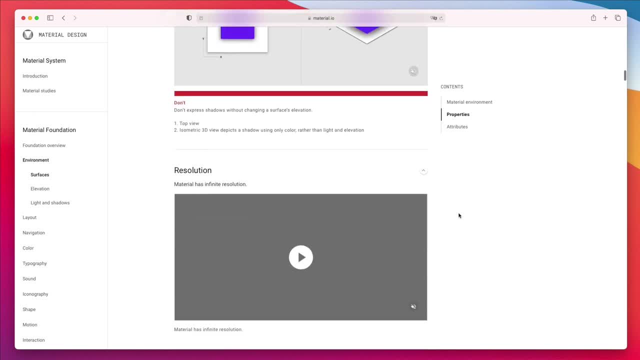 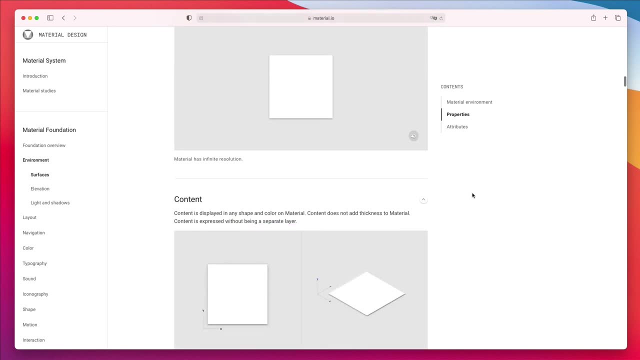 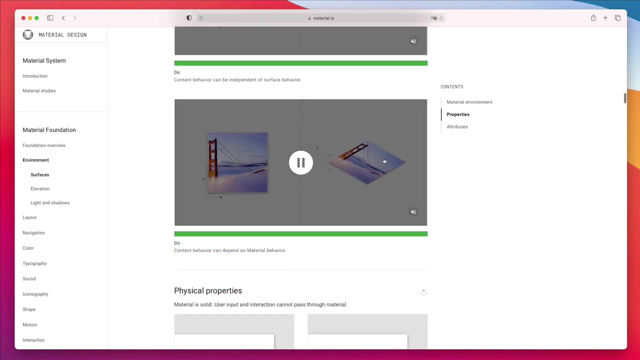 out there And these are things which are going to help you level up really fast. if you just take a moment and you have a look at these resources Now, they're also really easy to understand And they're also interactive. So in my personal opinion, they're better than most books and even courses out there. So it's definitely a really good investment of your time to just go through these Now. there is a lot in the Google. 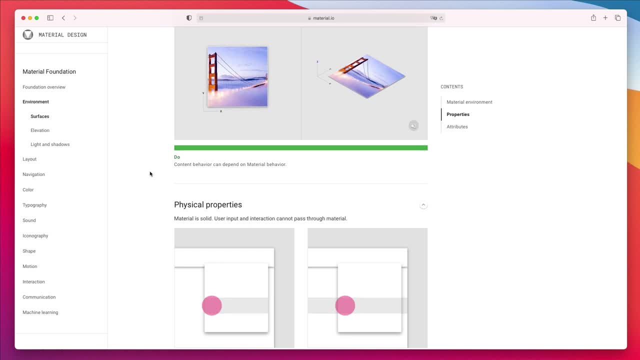 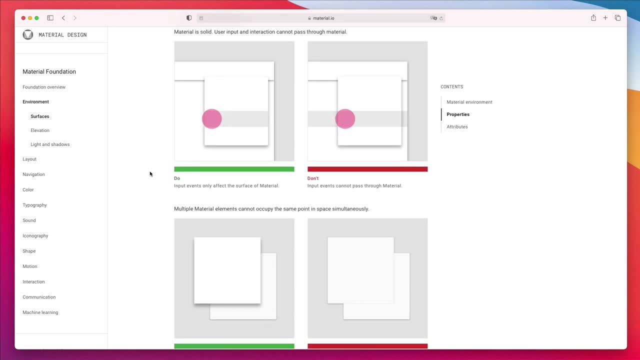 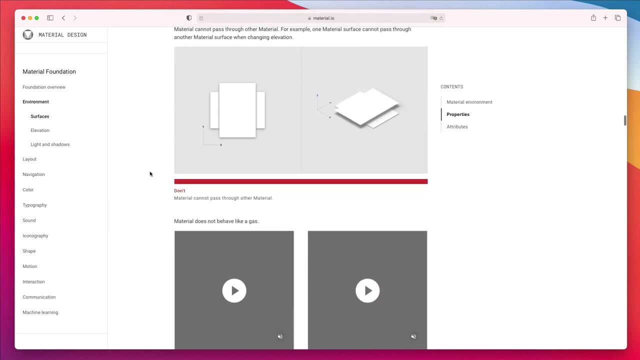 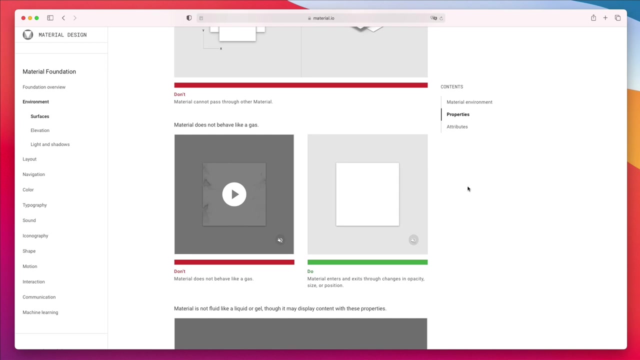 material design guidelines, So treat it as a course or a book. you're not going to be expected to go through all this in one single video or one single session. it's going to take time, But this is one of my best recommendations that I always give it to my coaching students is, that is, to actually go ahead and study these different elements and concepts of Google material design, Since most people think that. 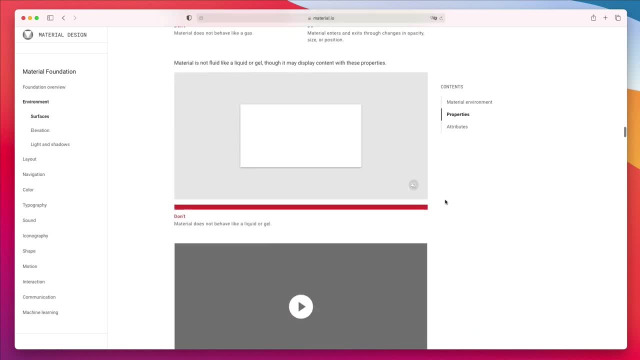 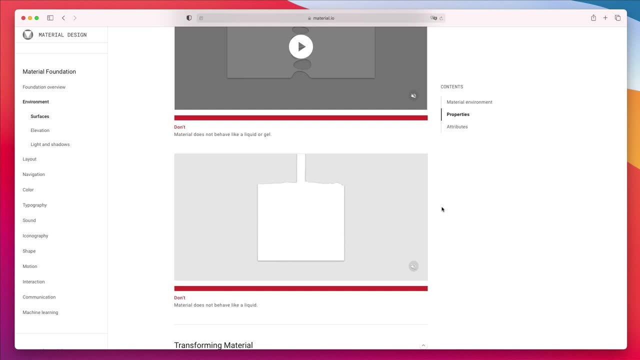 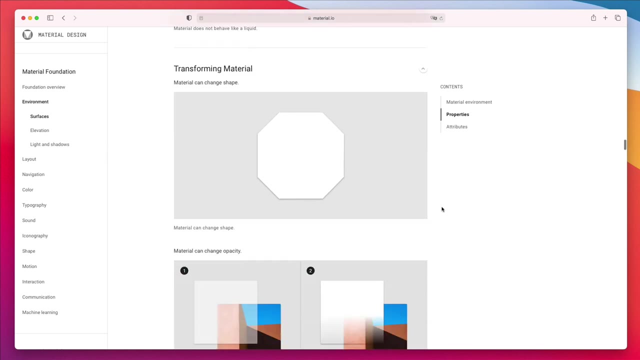 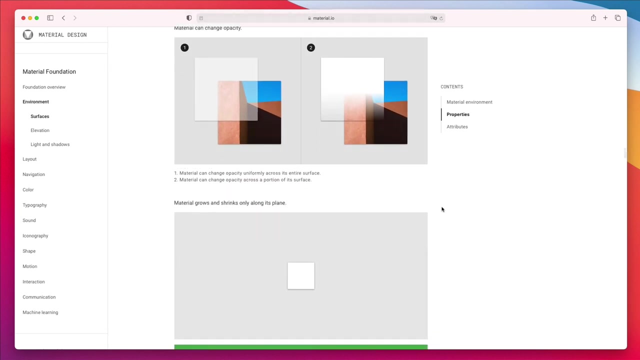 great UI UX design is just a matter of visual aesthetics and you know color combinations and finding the right font, But the reality is that whenever you see a great UI UX design experience, each and every one of those elements have a logic behind it. So you're not going to be naturally drawn to a solution which is not really fulfilling some key criteria, which are actually: 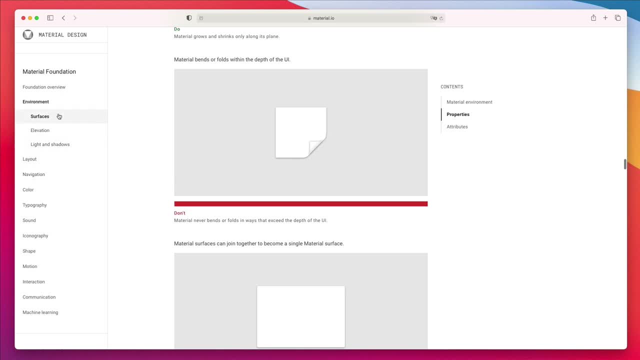 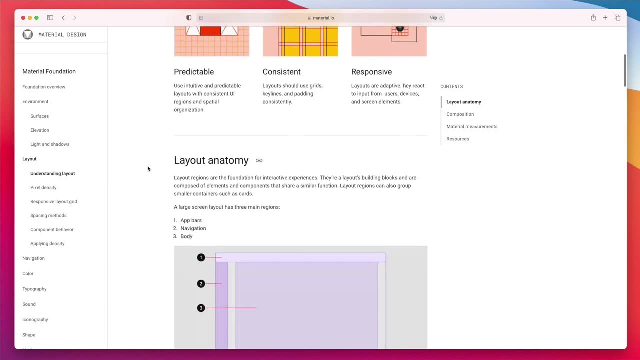 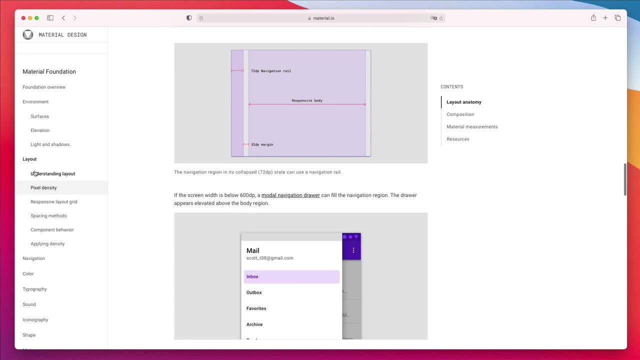 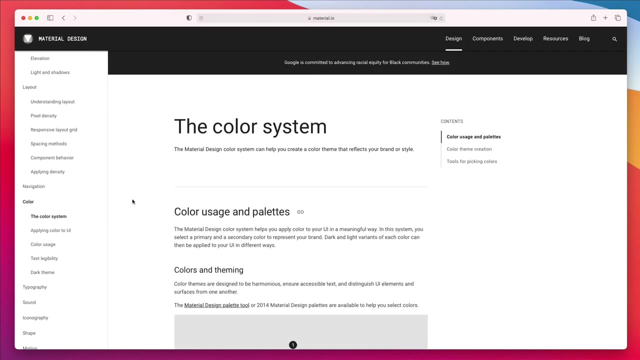 important explained over here And, as a brief overview, I want to really have you focus on things like the layout, which is really important, And some of these elements are not going to be maybe- maybe they're going to be like too granular and stuff, But I would definitely suggest to go through the layout and things like the colors and the navigation and the typography, because those are going to be really useful as well. 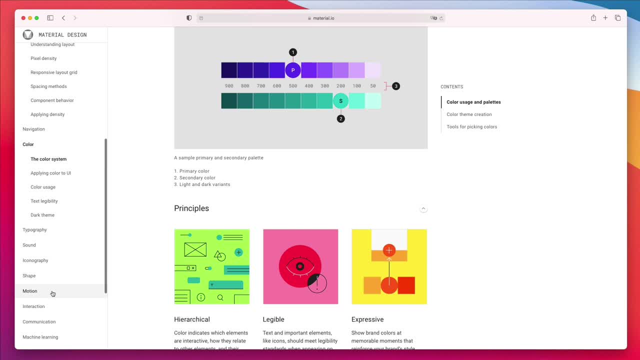 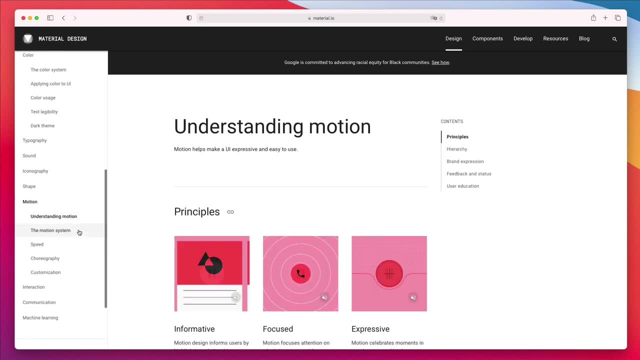 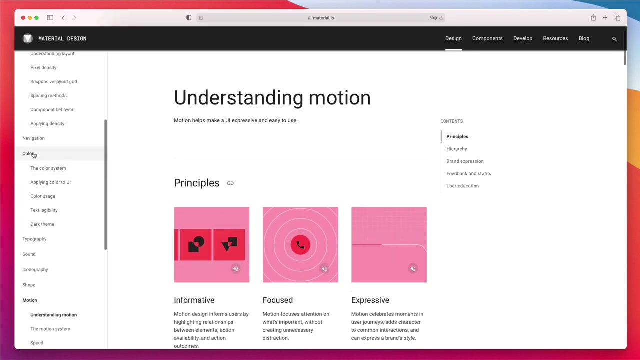 as iconography and shape. Now, if you're going to really take it one step further, you can go and have a look at the motion and even the interaction sections, But in my opinion that's a smaller portion of what the UI UX designer do. especially if you're just starting out, some of these sections might be quite advanced. So if you're just starting out in UI UX design, I would- I would highly recommend.